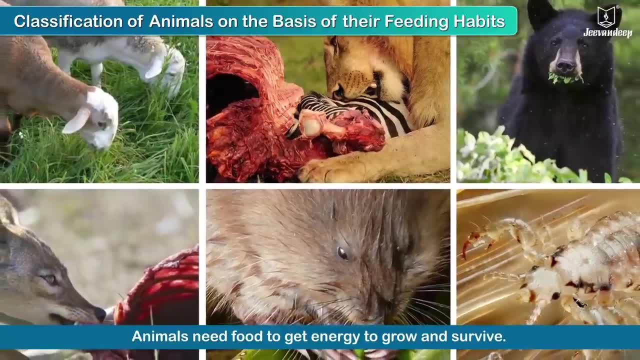 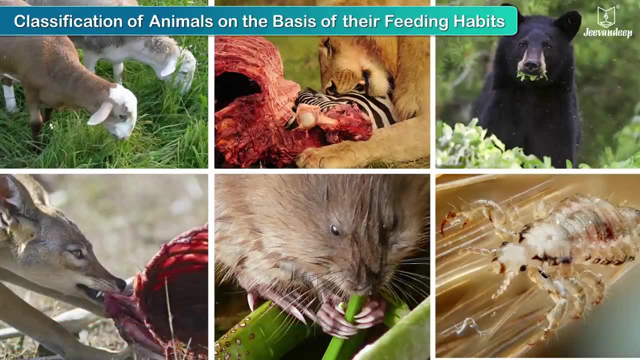 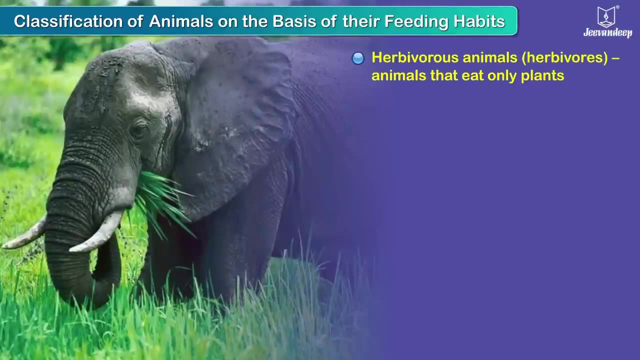 Like all living beings, animals do need food to get energy and survive. Animals can be classified on the basis of their feeding habits as herbivorous animals or herbivores are the animals that eat only plants. Carnivorous animals or carnivores are the animals that provide food, water and even. 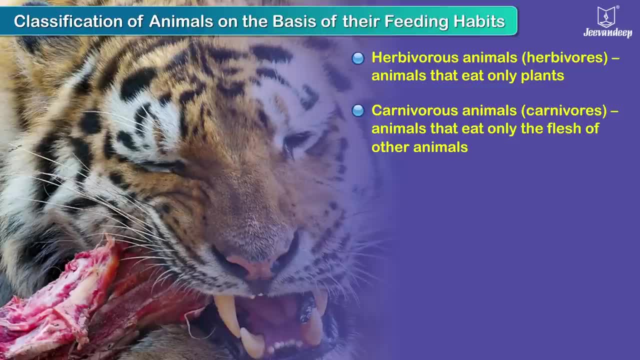 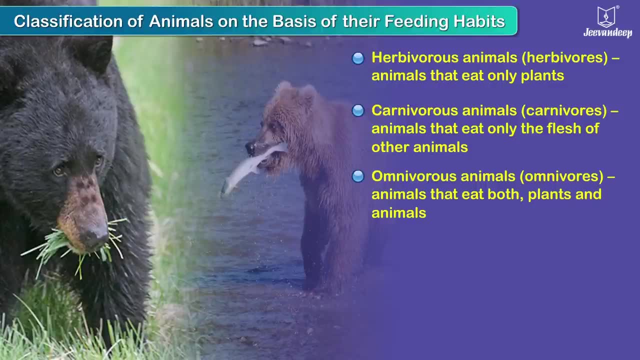 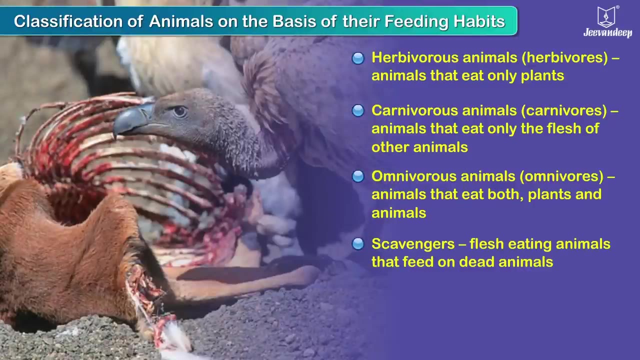 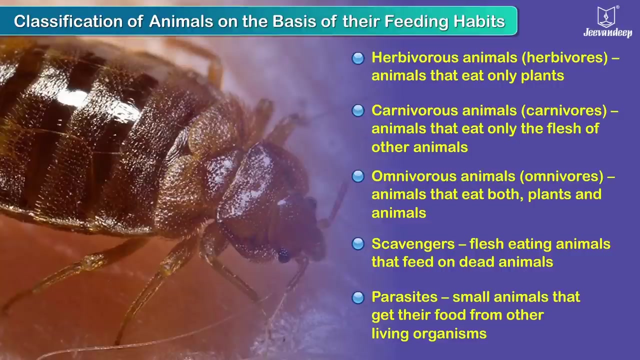 food for animals that eat only the flesh of other animals. Omnivores are the animals that eat both plants and animals. Scavengers are the flesh-eating animals that feed on dead animals. Parasites are some small animals that get their food from other living. 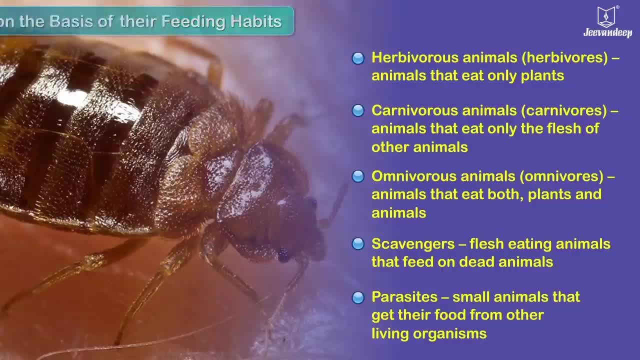 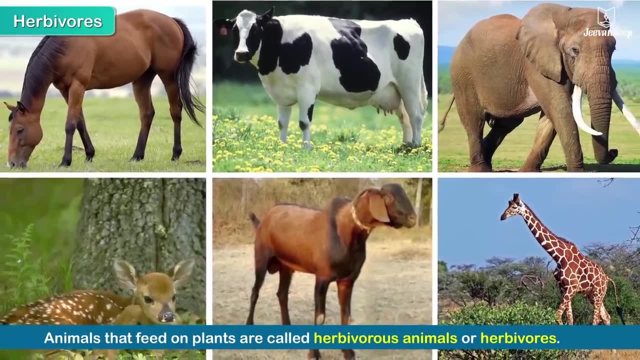 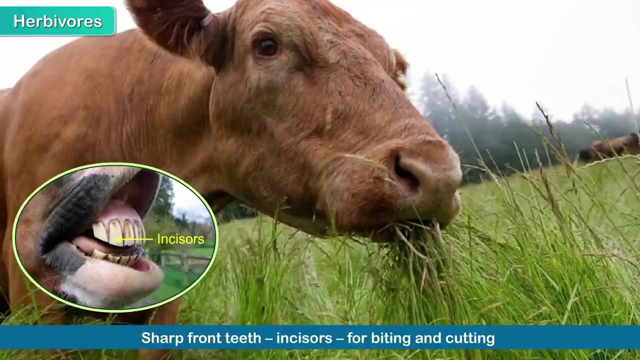 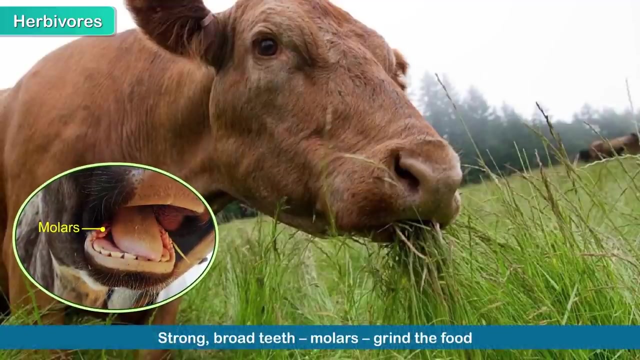 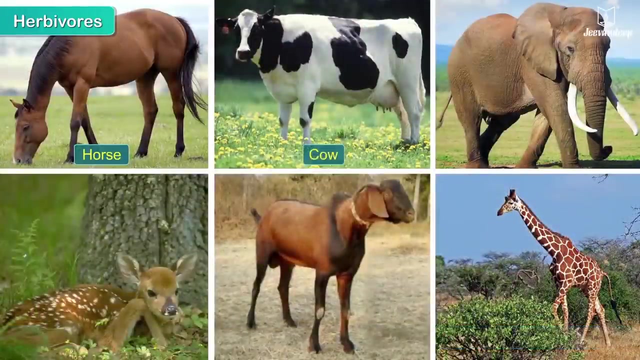 organisms Herbivores. Animals that feed on plants are called herbivorous animals or herbivores. They have sharp front teeth, called incisors for biting and cutting and very strong, broad teeth called molars, to grind the food. Horses, cows, elephants, deer goats, giraffes are some herbivorous animals. 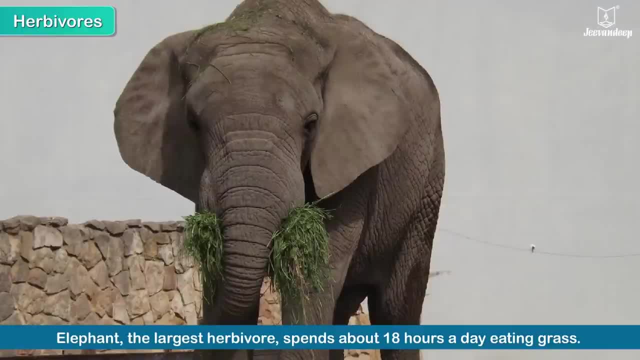 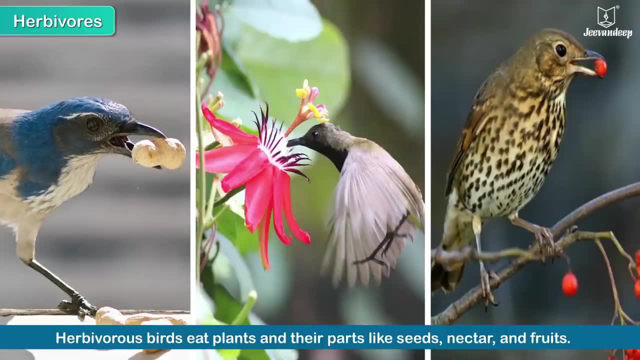 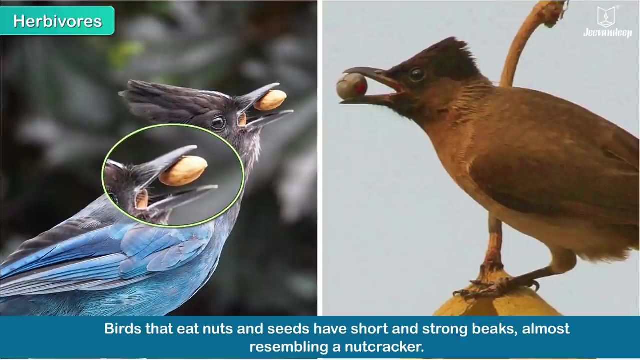 Elephant, the largest herbivore, spends about 18 hours a day eating grass. Herbivorous birds eat plants and their parts, like seeds, nectar and fruits. Birds that eat nuts and seeds have short, and strong beaks, almost resembling a nutcracker. 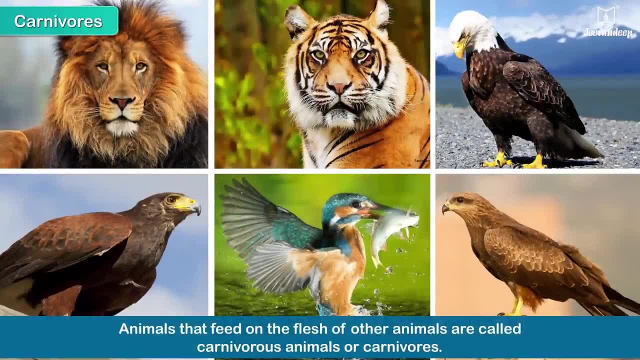 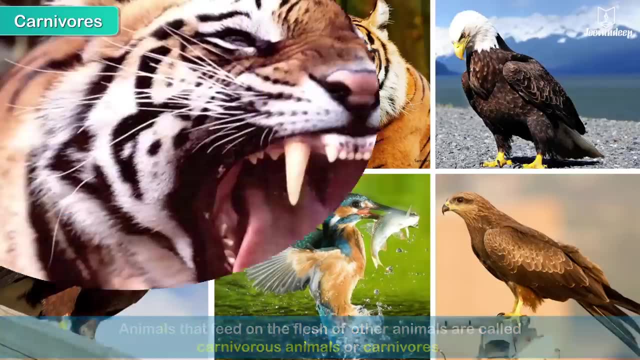 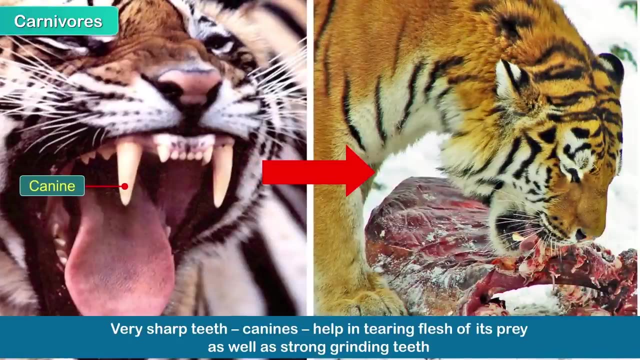 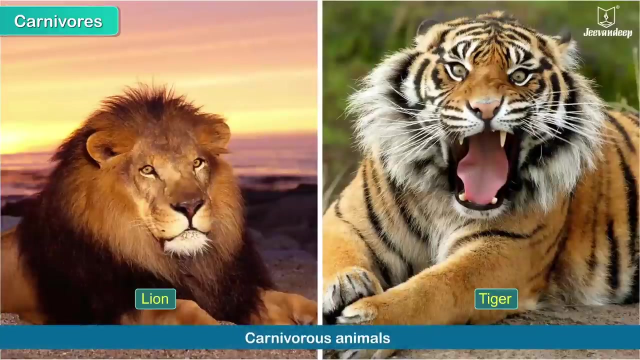 Carnivores: Animals that feed on the flesh of other animals are called carnivorous animals or carnivores. These have very sharp teeth, called canines, that help in tearing the flesh of its prey, As well as strong grinding teeth. Lions and tigers are some carnivorous animals. 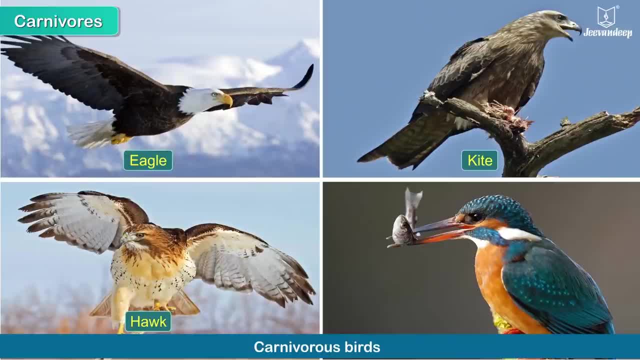 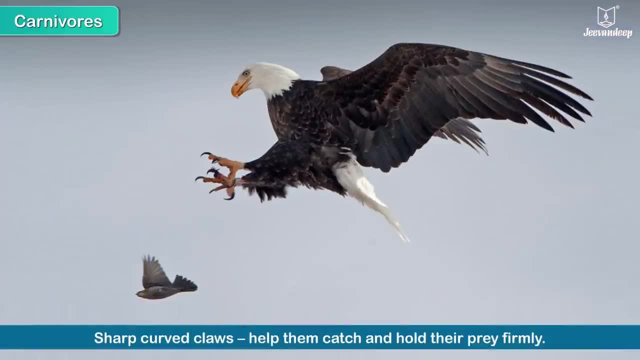 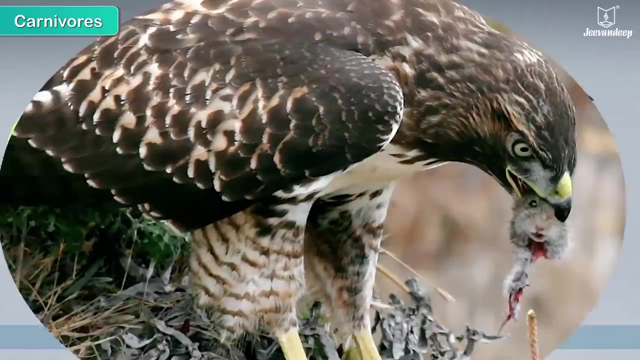 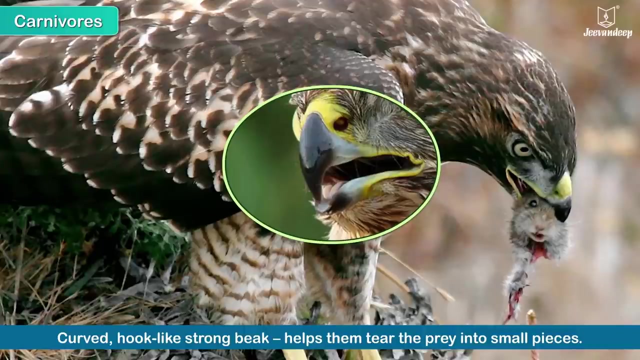 while eagles, hawks, kites and kingfishers are some carnivorous birds. Their sharp, curved claws help them catch and hold their prey firmly. They also have a curved hook-like strong beak which helps them tear the prey into small pieces. 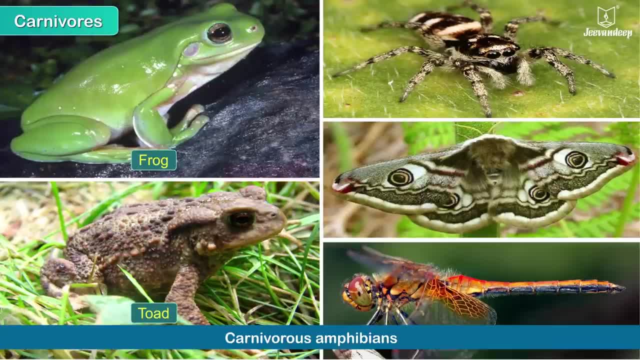 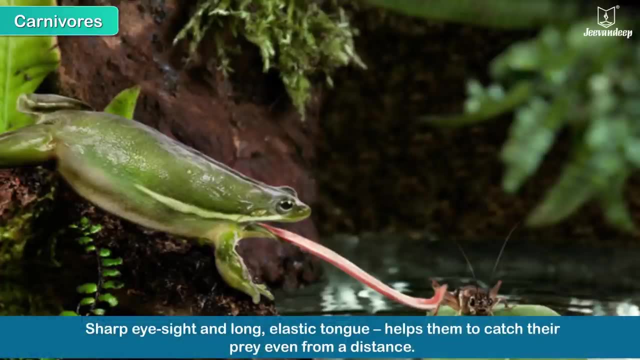 Carnivorous amphibians like frogs and toads feed on spiders, moths, dragonflies and many other insects. Their sharp eyesight and long, elastic tongue helps them to catch their prey even from a distance. How to catch a carnivore? 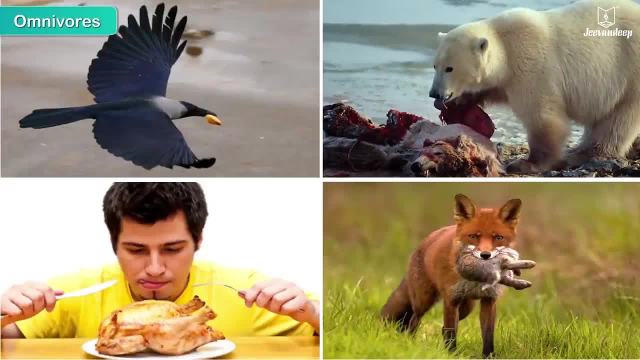 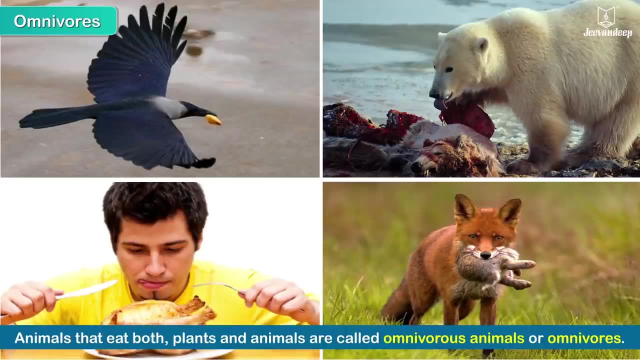 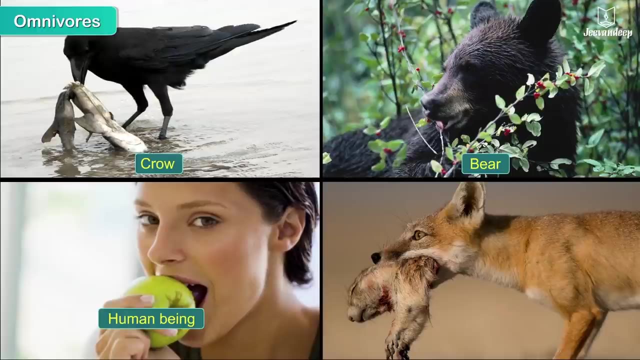 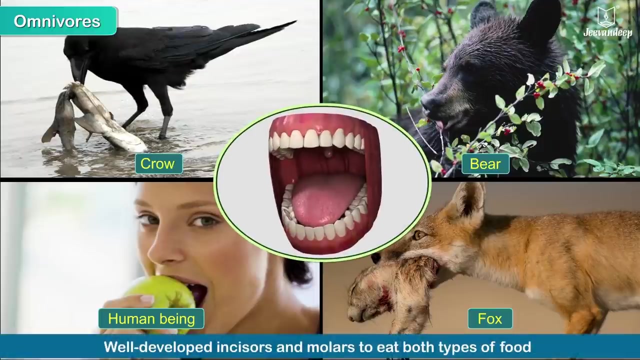 Animals that eat both are called omnivorous animals or omnivores. Crows, bears, human beings and foxes are some omnivores. Omnivores have well-developed incisors and molars to eat both types of food- The carnivore. 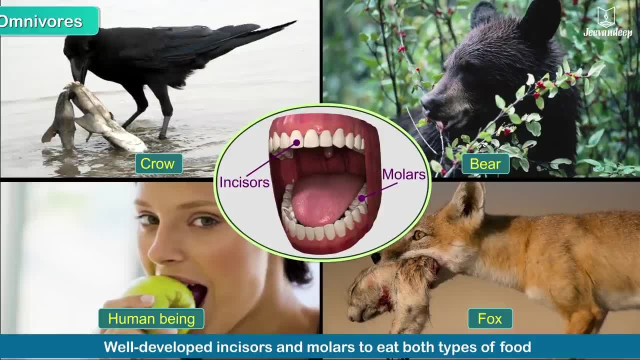 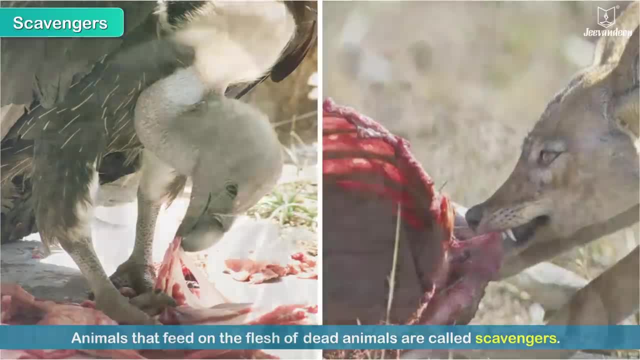 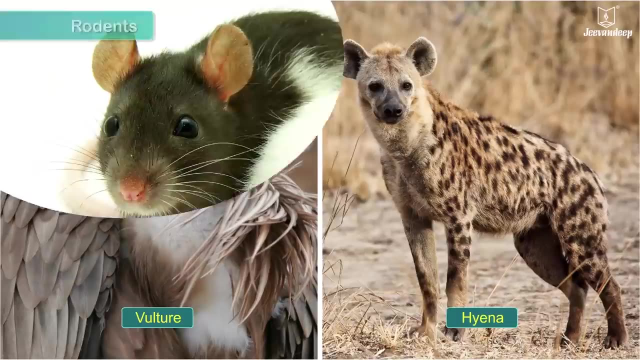 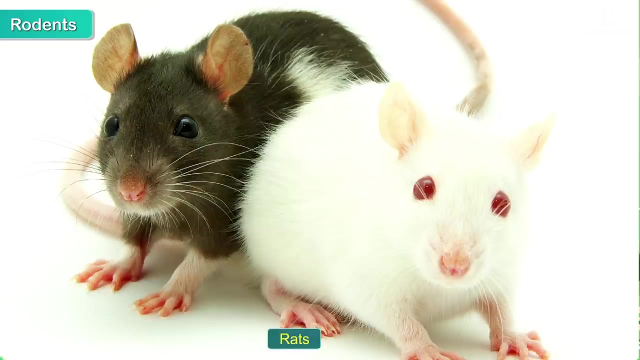 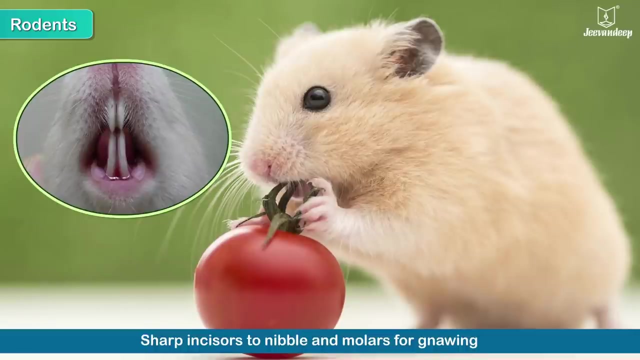 is a carnivorous animal and is known to watch people eating their prey When they are eating of food. scavengers: these are animals that feed on the flesh of dead animals. vulture hyenas are some scavengers. rodents: many rodents, like rats, are able to eat almost anything. they have sharp incisors to nibble and molars for. 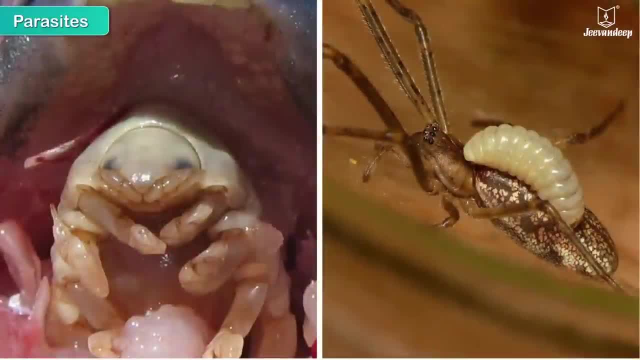 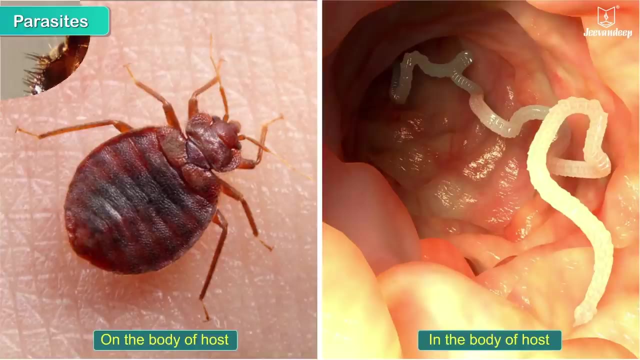 knowing parasites. some small animals get their food from other living organisms. they may live on or inside the body of their host. fleas and lice live on the host body, inside the host battery or food sheath and intestines. the host is Amyph Straus. those qui converter or birds and animals recur하기, they become 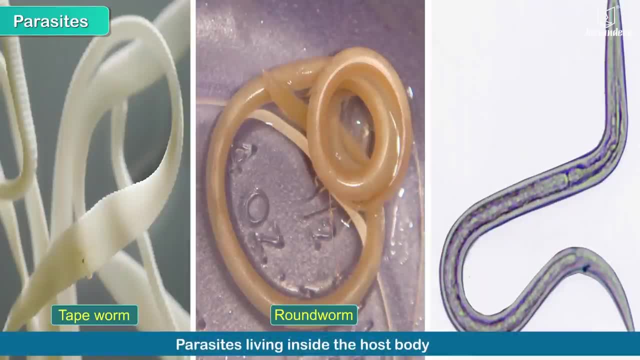 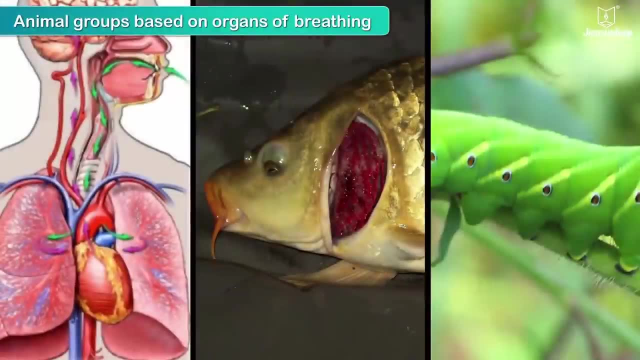 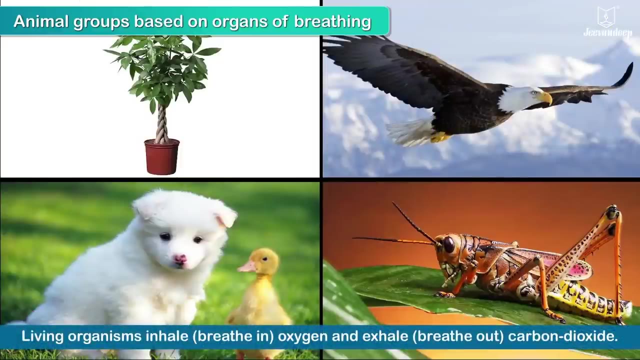 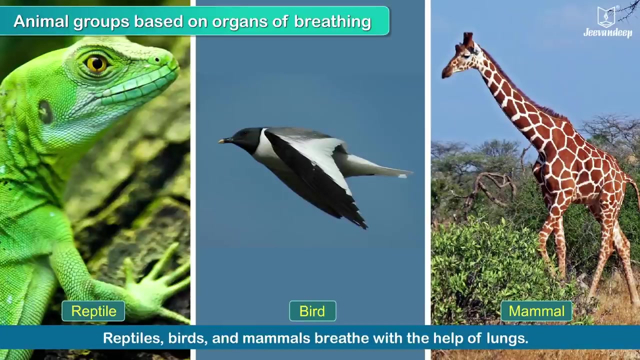 while tapeworm, roundworm and hookworm live inside it. animal groups based on organs of breathing- all living organisms- inhale or breathe in oxygen and exhale or breathe out carbon dioxide. reptiles, birds and mammals breathe with the help of lungs. however, they have different organs for breathing: breathing in. 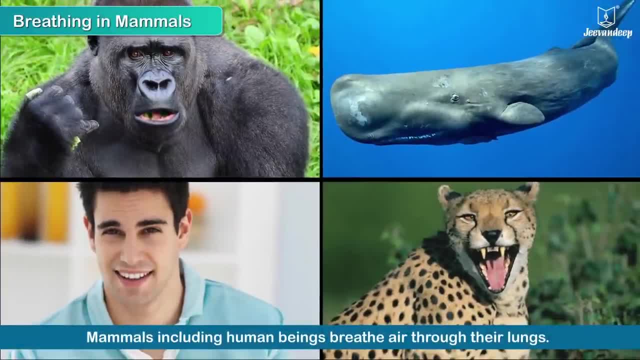 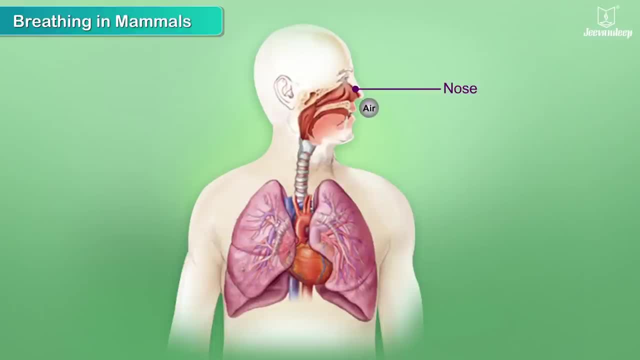 mammals. mammals, including human beings, breathe air through their lungs. air is taken in through the nose and mouth and down the airway that is the trachea, or windpipe, into the lungs. the carbon dioxide is then thrown out of the lungs and exhaled through the mouth. 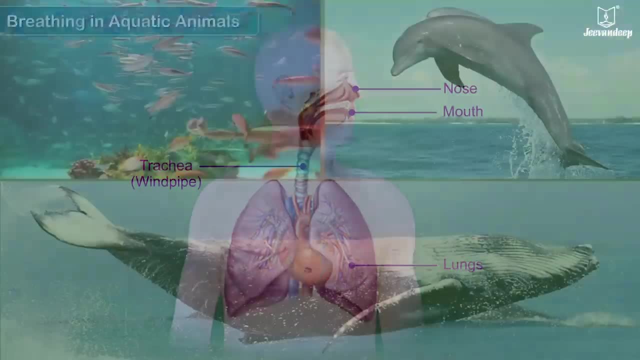 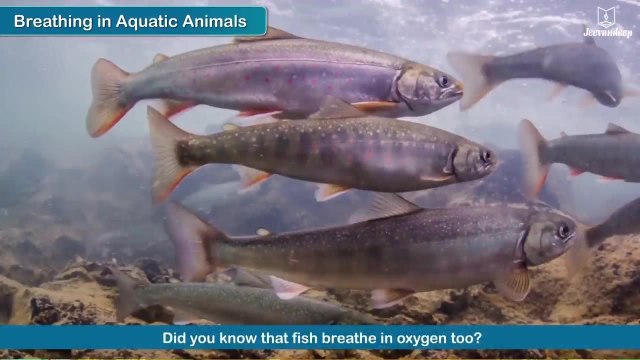 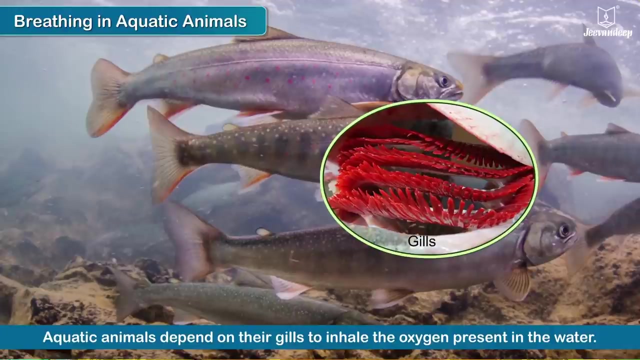 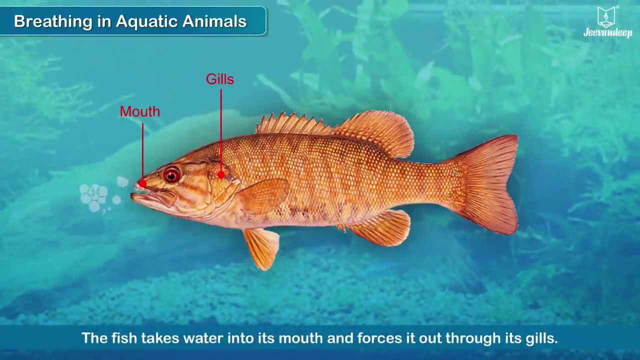 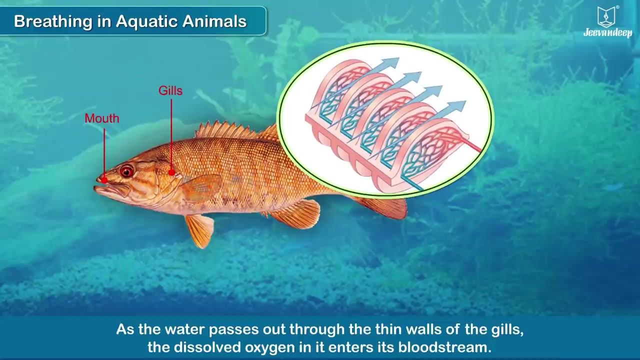 or nose breathing in aquatic animals. did you know that fish breathe in oxygen too? you also know, for different organisms come into the hot water populations. they depend on their breathing organ- the girls- to inhale the oxygen present in the water. the Fish takes water into its mouth and forces it out through its 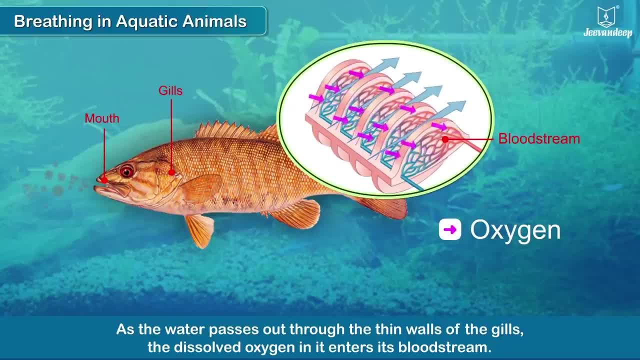 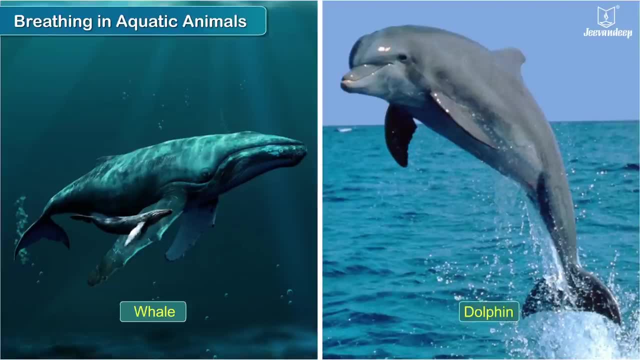 gills. as the water passes out through the thin walls of the gills, the dissolved oxygen in it enters its bloodstream. There are, however, exceptions, like devices among other Sichtżyć, Custom, Neut, Sesame and Hyahth equipment, whales and dolphins. they breathe in the oxygen present in the air through their 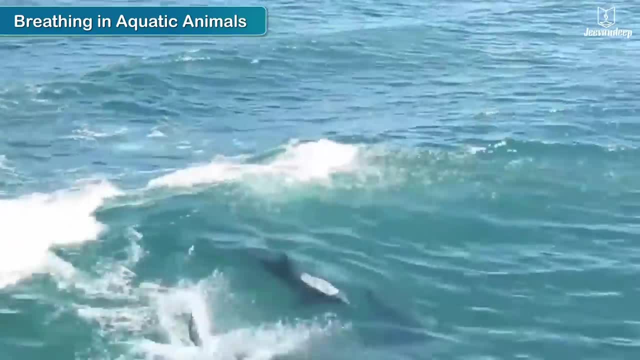 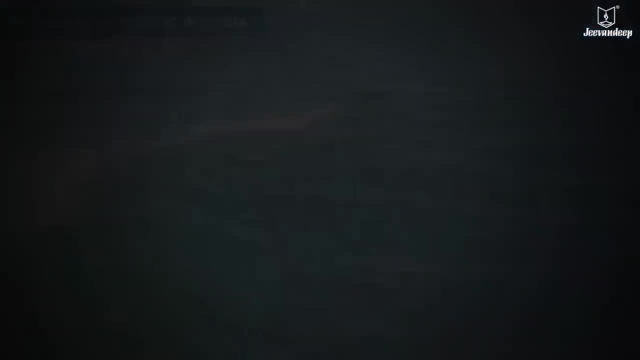 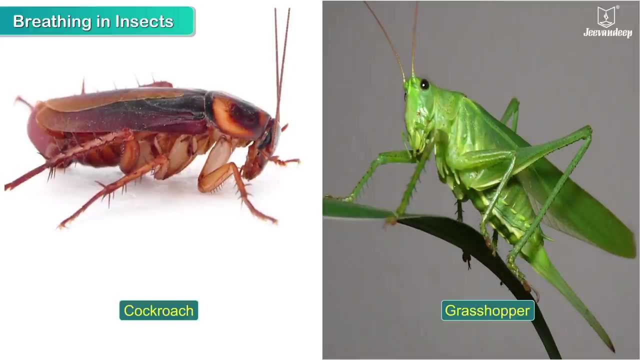 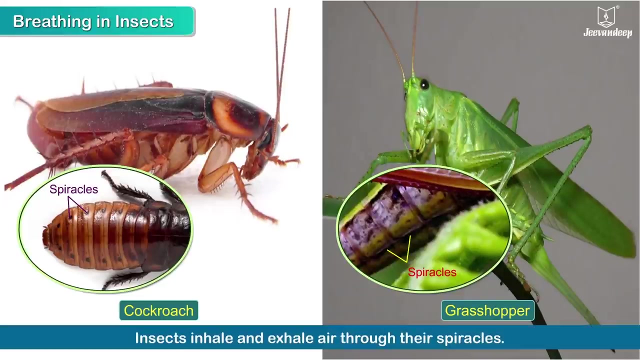 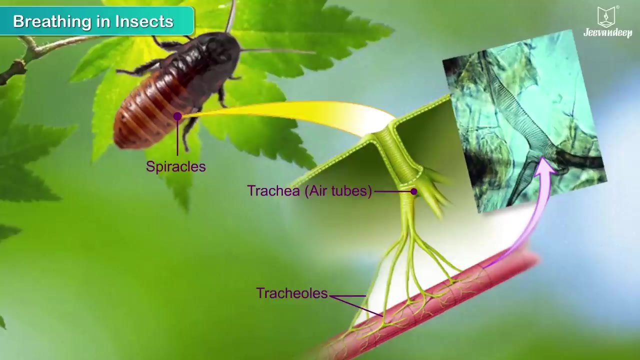 lungs. they do this by coming up to the water surface breathing in insects. insects such as cockroaches and grasshoppers have very small openings on their bodies, called spiracles, through which they inhale and exhale air. the spiracles open into a network of air tubes inside the body called trachea. 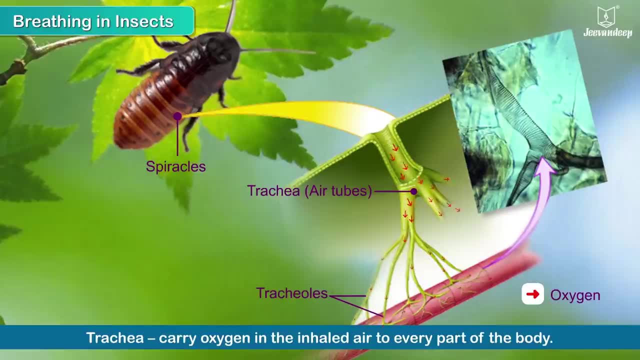 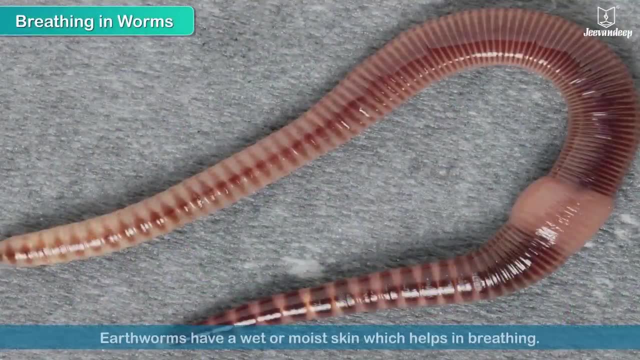 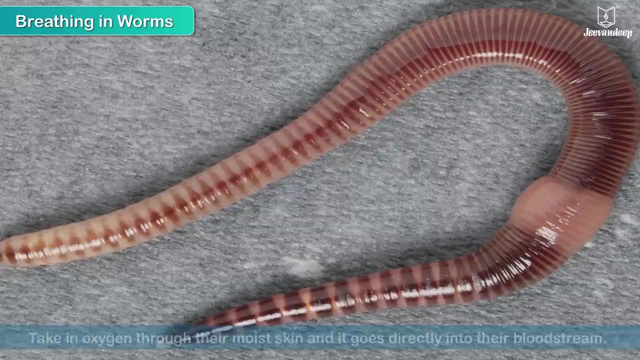 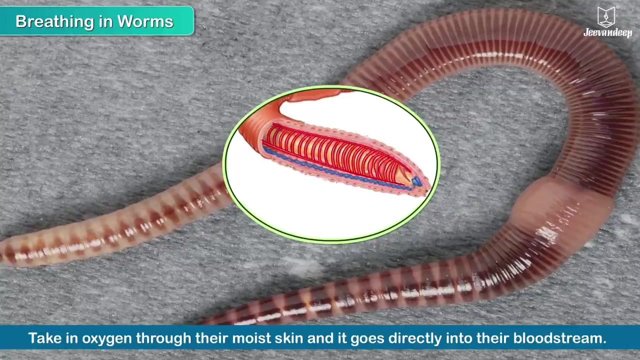 which carry oxygen in the inhaled air to every part of the body breathing in worms. earthworms have a wet or moist skin which helps in breathing. They take in oxygen through this moist skin and it goes directly into their bloodstream. That is why earthworms are generally seen. 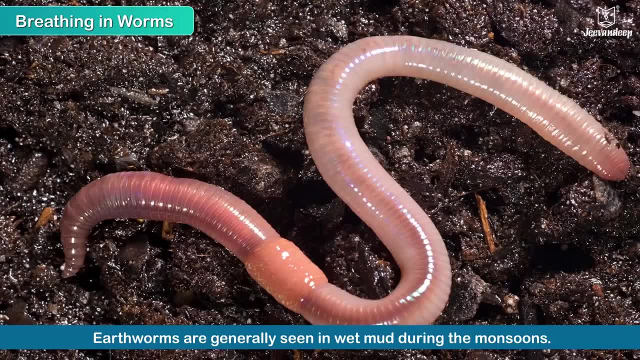 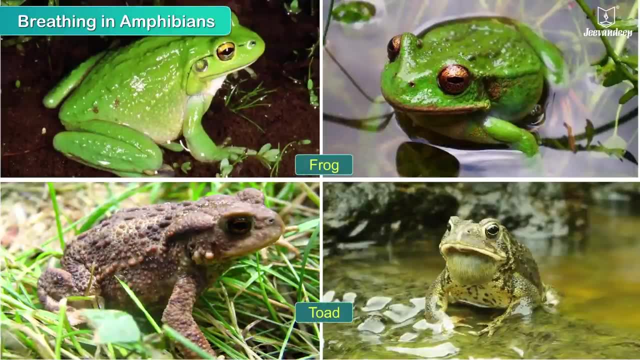 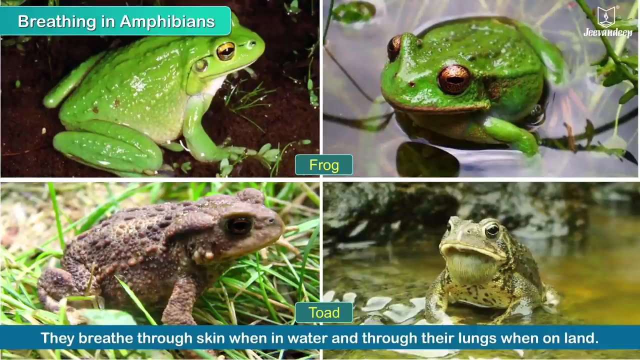 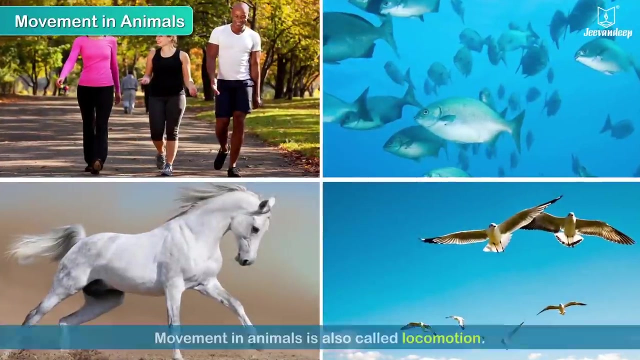 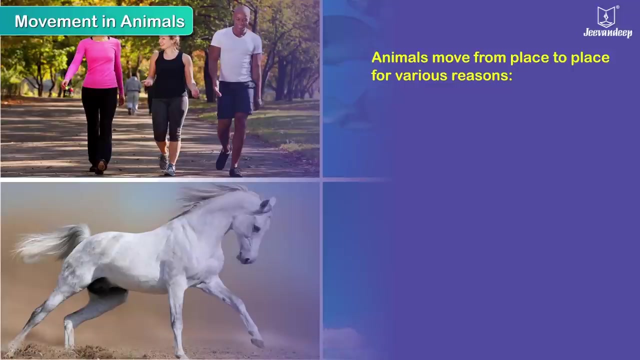 in wet mud during the monsoons, Even in amphibians. frogs and toads live on land as well as in water. They breathe through skin when in water and through their lungs when on land. Movement in Animals. Movement in animals is also called locomotion. Animals move from place to place for various 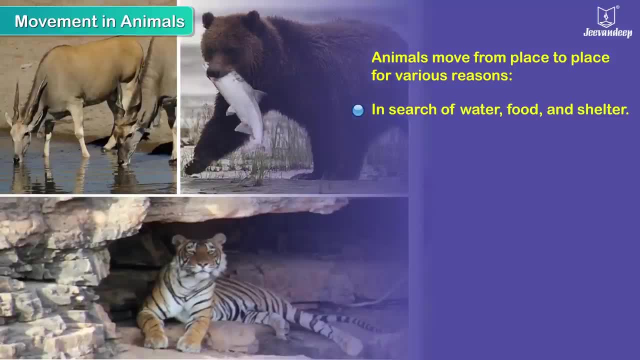 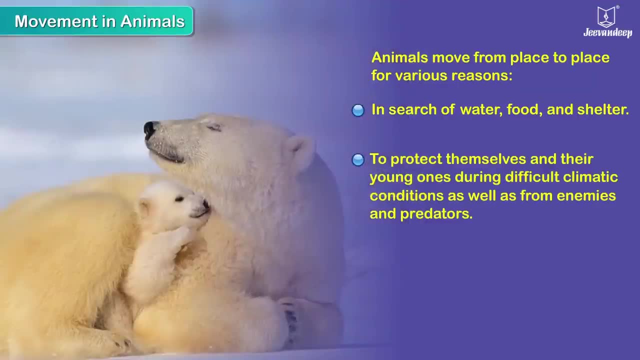 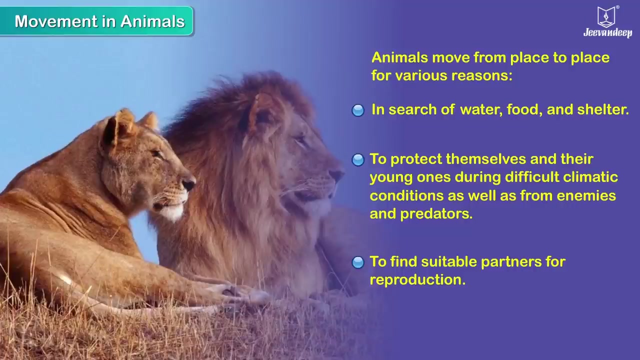 reasons: In search of water, food and shelter, To protect themselves and their young ones during difficult climatic conditions, as well as from enemies and predators, To find suitable partners for reproduction. Movement in Terrestrial ie Land Animals. Movement in Terrestrial ie Land Animals. 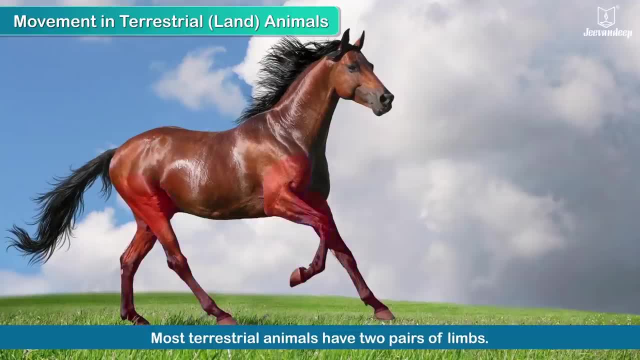 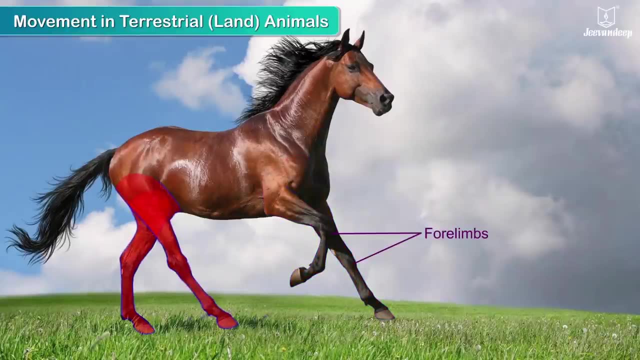 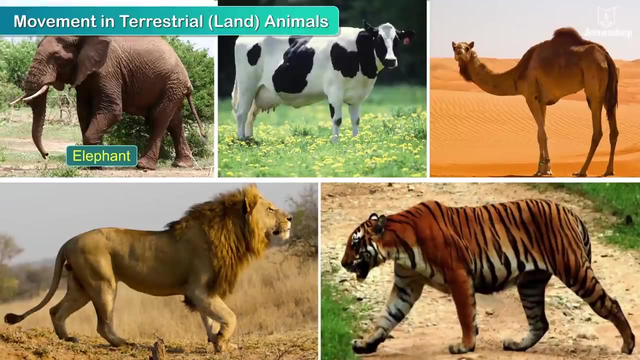 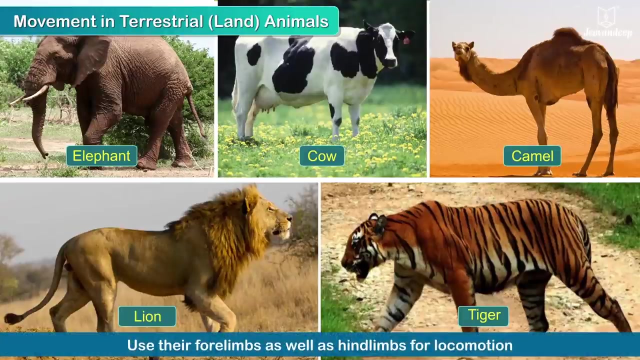 Movement in Terrestrial, ie Land Animals. Most terrestrial animals have two pairs of limbs. The front ones are called forelimbs, while the rare ones are called hindlimbs. nurse animals are called hindlimbs or hindlines. Animals such as elephants, cows, camels, lions, tigers use their forelimbs as well as hindlimbs. 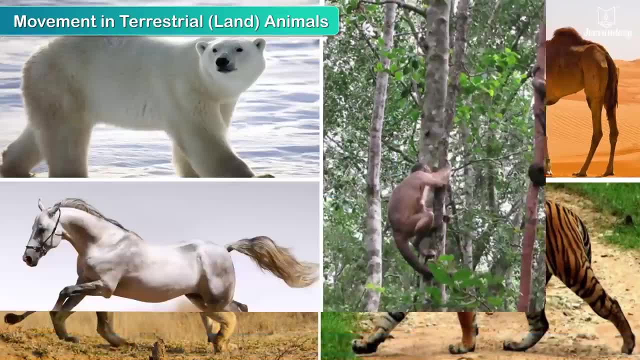 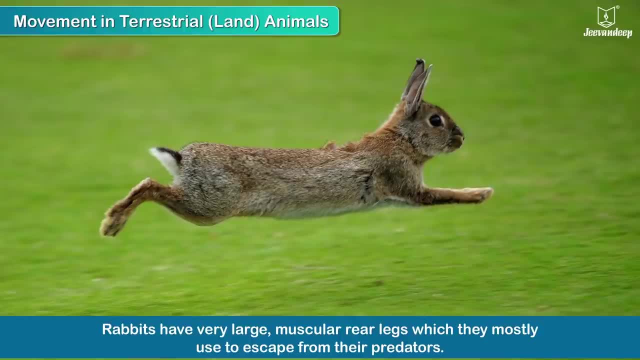 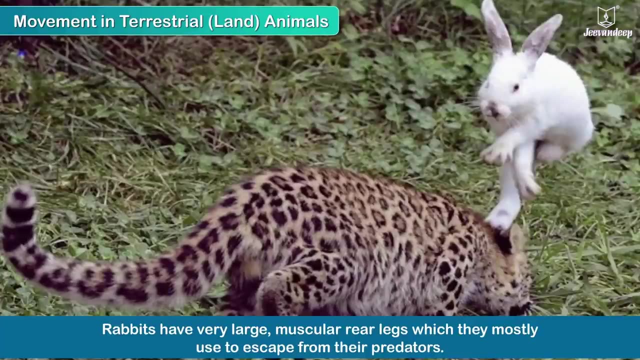 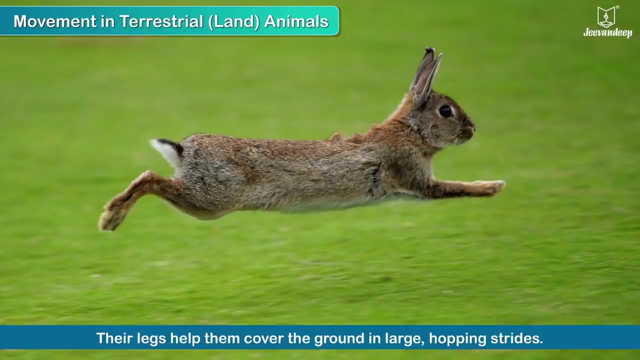 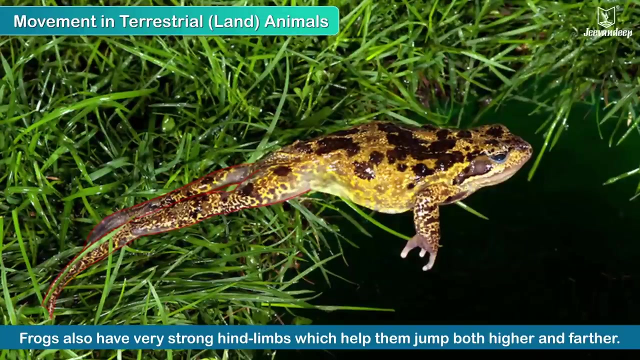 for locomotion Movement in Mouth, such as walking, running or climbing. Rabbits have very large, muscular, rare legs which they mostly use to escape from their predators. Their legs help them cover the ground in large hopping strides. Snakes also have very strong hind limbs which help them jump both higher and farther. 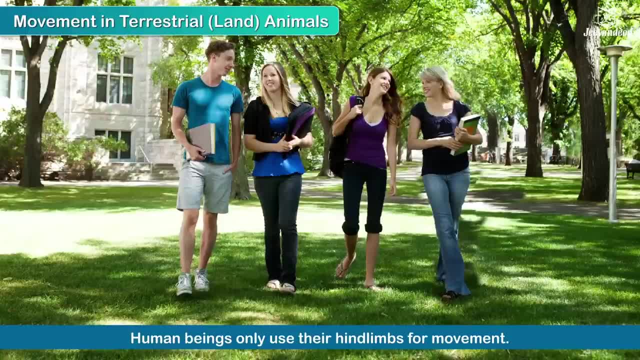 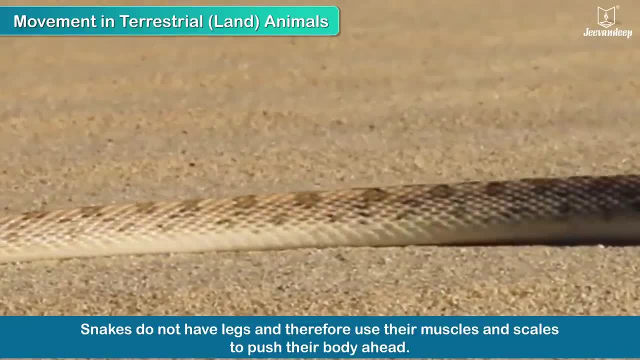 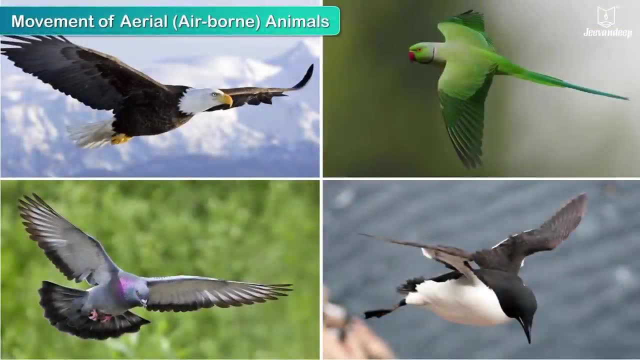 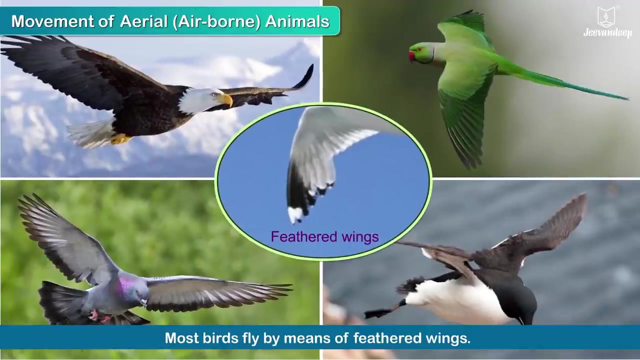 Human beings only use their hind limbs for movement. Snakes do not have legs and therefore use their muscles and scales to push their body ahead. Movement in Aerials, ie Air-Born Animals. 1. Feathered Wings: Most birds fly by means of feathered wings. 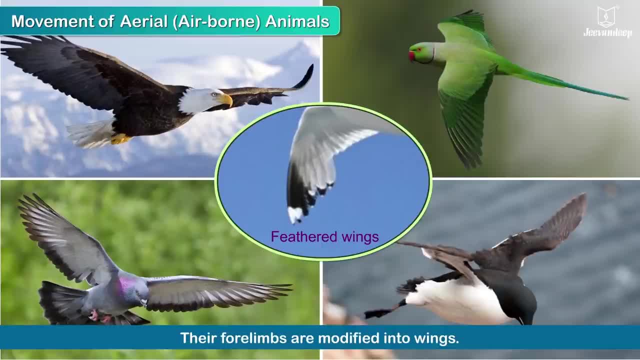 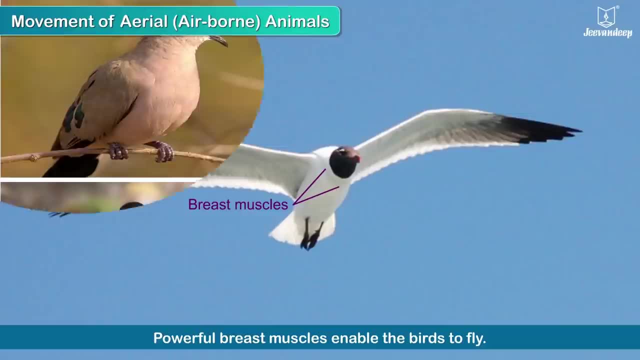 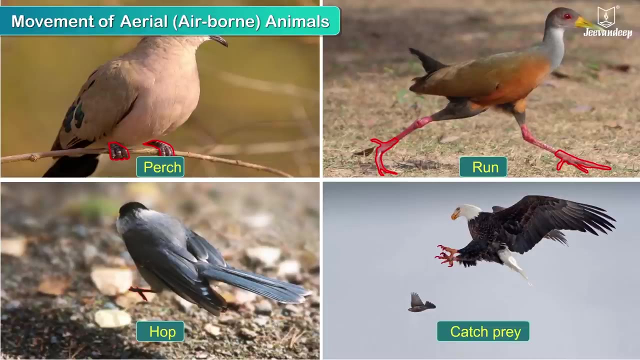 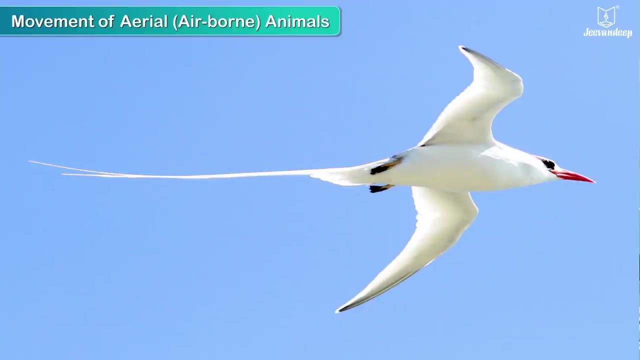 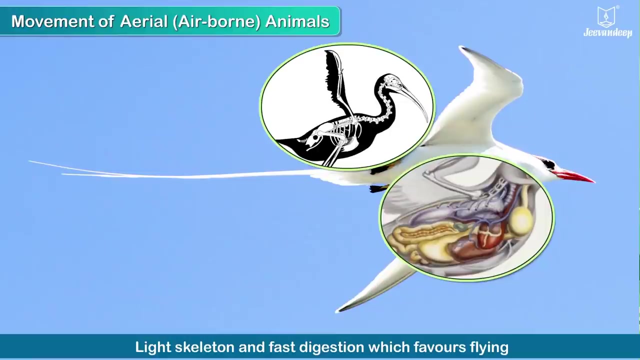 Their forelimbs are modified into wings. They have powerful pressed muscles which help them fly in air. Their hind limbs help them to perch, hop, run and catch prey. Tails also help them direct the fore. 2. the flight birds have a very light skeleton and fast digestion which favors flying bats also fly. 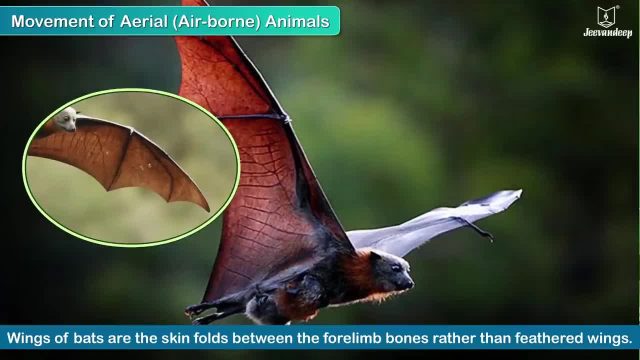 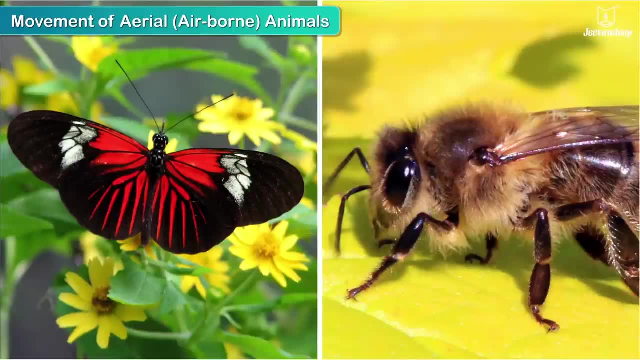 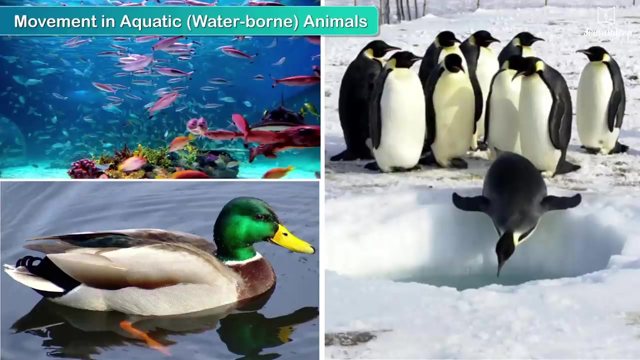 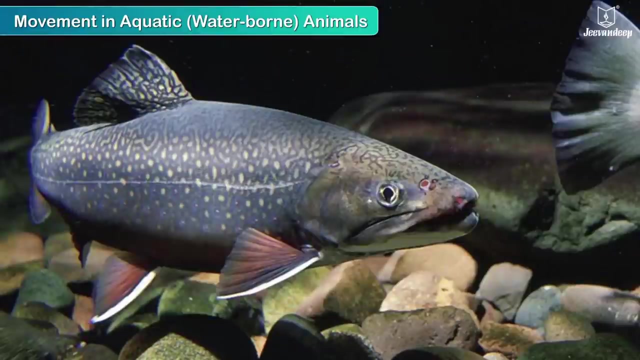 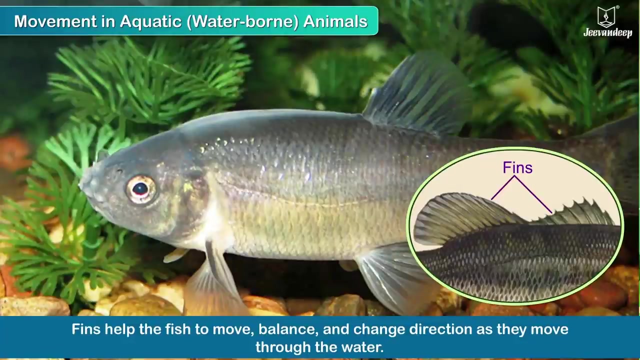 but their wings are actually the skin folds between the four limb bones, rather than feathered wings. insects like butterflies, bees etc. have thin membranes which helped them fly movement in aquatic, that is, waterborne animals. fish are an excellent example of adaptation in animals. their streamlined body helps them swim in water. their fins help to move, balance and change direction as 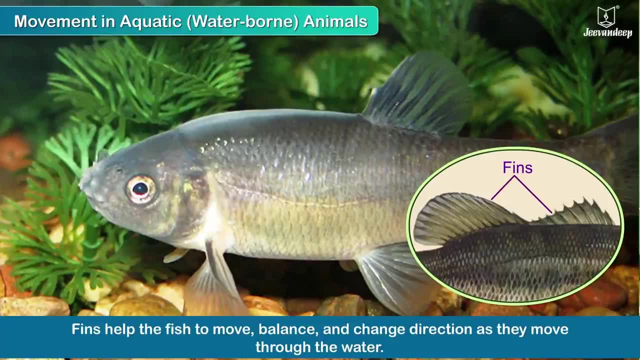 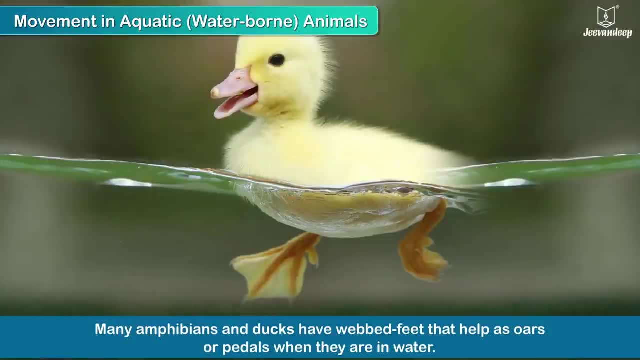 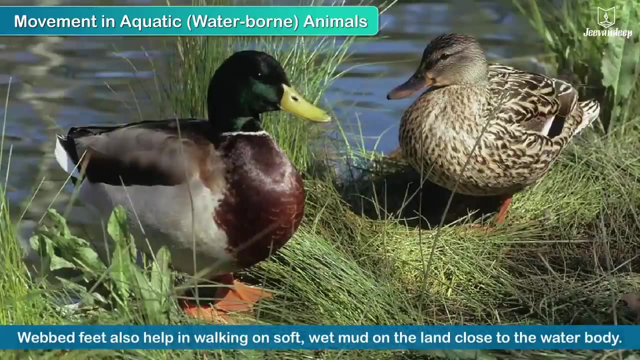 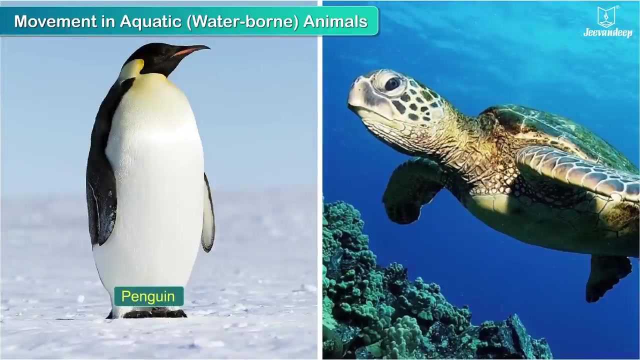 they move through the water. many amphibians and ducks have wept feet, since they held them as oars or pedals when they are in the water or to walk on the soft, wet mud when they are on the land close to the water body. penguins, that is, aquatic flightless birds, as well as sea turtles, have their four limbs in.